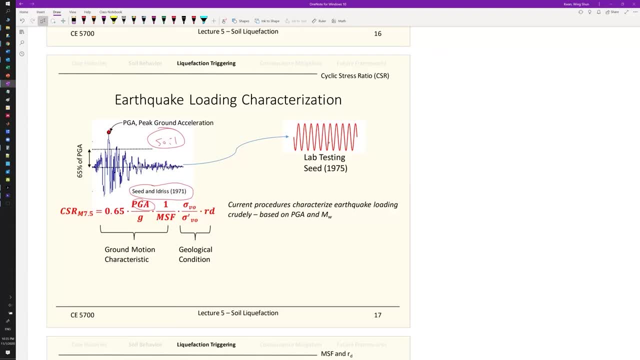 by the g over here, and then you times upon six, five uh derived by the magnetic scaling factors- we will talk about this like uh, uh, you know. next slide and then times the uh, total stress derived by vertical stress and also divide multiplied by a depth of reductions of factors we will talk about. 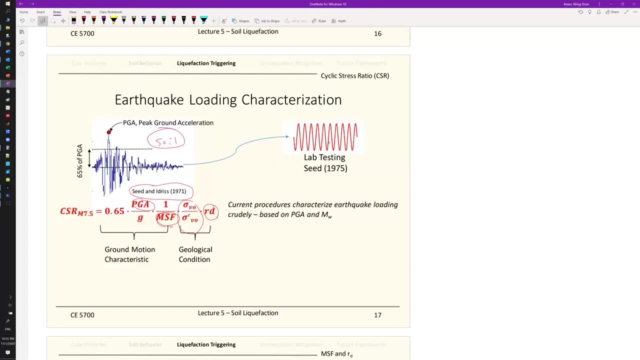 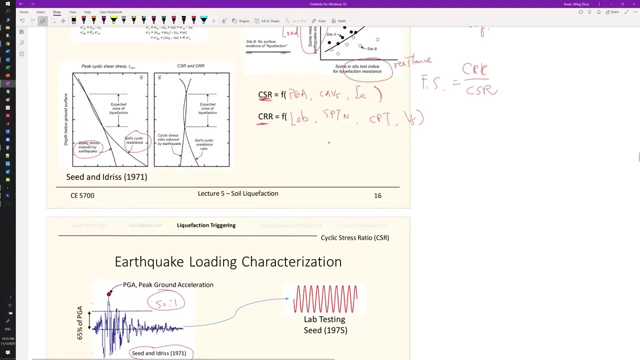 this along with the ms alpha in the next slide. so pretty much this is a framework for uh based on: based on uh, the uh assertion time history that you design for can convert it to become a psychic stress ratios. then you can do your site specific: uh, uh liquid fractions, uh- irradiation. so therefore, so this: 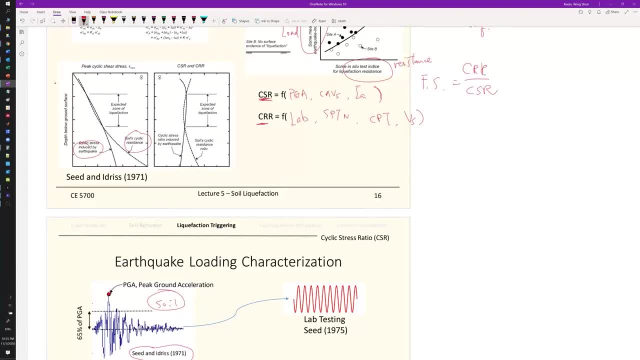 pretty much like. it's kind of like a screening tool people do once they have their site specific data. you want to see whether uh, like you know, means like cpt or spt data. you want to see uh have a quick check. uh, rather like you know, you see. 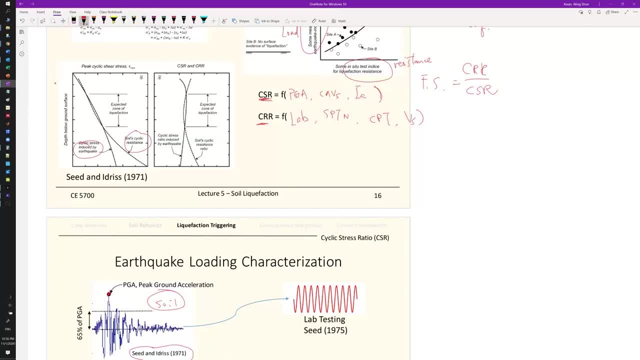 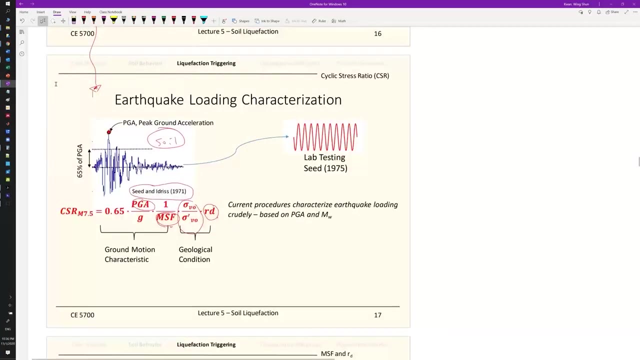 your site is susceptible for other fractions to be happens, then you will calculate the csr based on these like ground motions. so this psychic stress ratios, you know this like a line here, pretty much just plot by that pop by, like the equations here, because, uh, now those two terms. 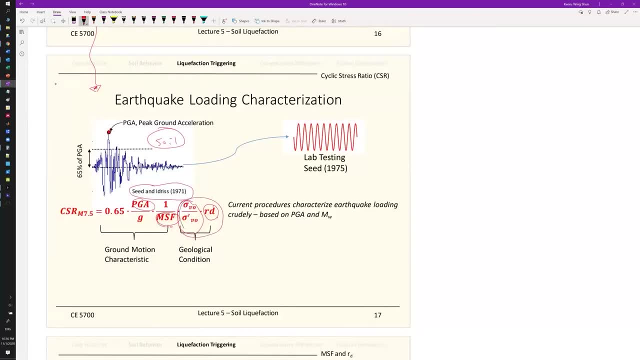 actually these three terms are function of that. so, uh, you can, you can uh from this depth and csr with these equations, because this is uh, this, this three terms, these are functions of uh, z the depth. so you can kind of like a plot out the uh, the curve there, the csr versus depth. 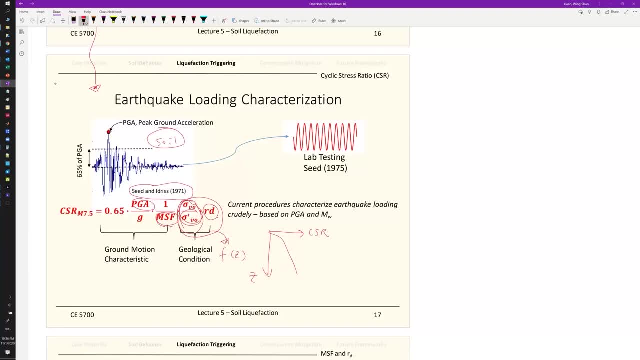 based on these equations, uh, provided you have already known your pga. so, uh, this, this framework, you realize that, uh, it has uh factors 0.65 y 0.65. you know that's based on the early work from a seed. uh, you know he has some work that like also convert uh, uh, a series of time history, uh into 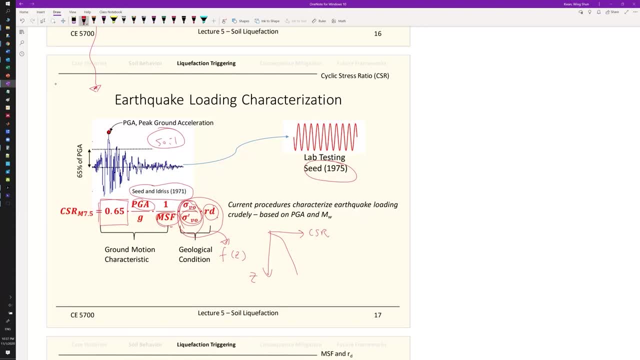 a series of harmonic motions such that, like you know uh he can uh more easy to uh try to model uh uh the earthly phenomenon in the lab, because, remember, back to the old days, it's not like uh quite possible to to input uh neurotic, uh axios whose time history with positions in the lap. but 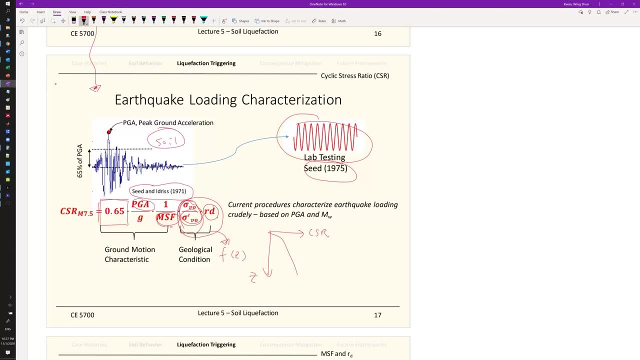 uh, harmonic science, uh forms, is doable through cyclic loading and actually it's more practical to use like a series of harmonic motions to represent a surface in time history. so, uh what? but like the seat 1975 uh work they had done, taking 65% of the PGA, and then convert that into a series of harmonic motions. so it's about 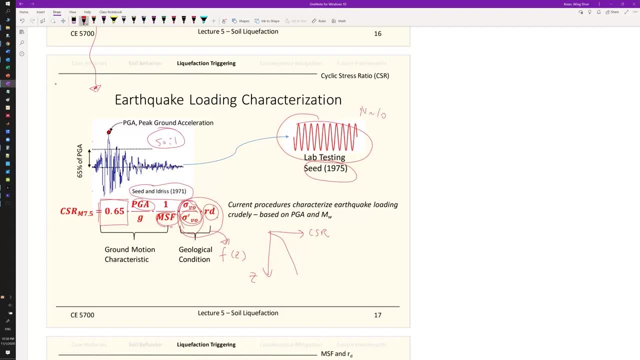 and it's about 10. so he he tried to represent our earthquake one motions by, you know, a series of like a 10 harmonic motions with amplitudes equals to 65% of the PGA. so that was, like you know, the laboratory modeling we're doing in the early days and we're we are still doing it. you. 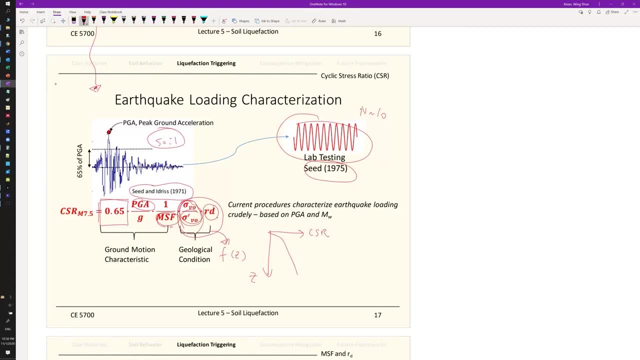 know today, in nowadays, so that's why you know this harry city is the father of judah earthquake engineering. he laid down the foundations for us to follow. but nowadays, like you know, it's possible to perform a real-time service and time history in the lab, but yet this work is only limited, like 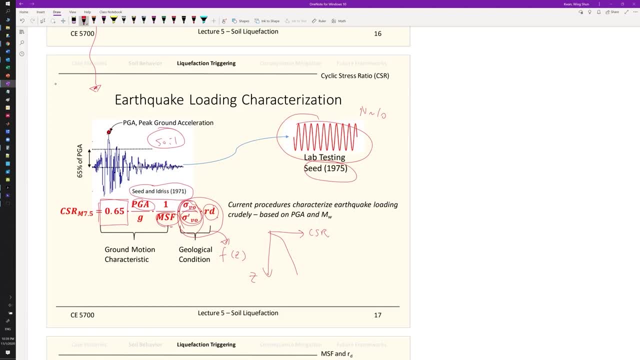 ukrainians able to do it more for research. in practice we still use like harmonic motions to move the model of your ground motions. so that's the equations to convert again, to convert a certain time history into a csr. and one more comments about this method. like you know, this the method. 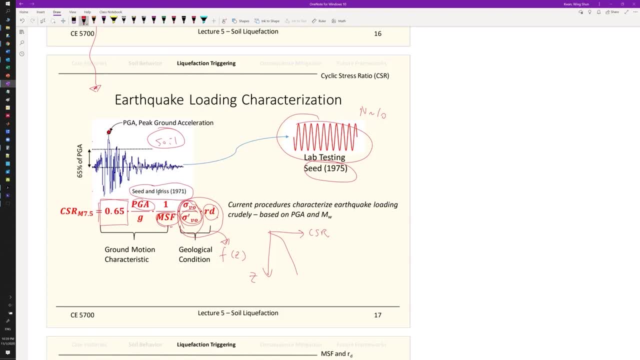 saying each method is a very good start, but for sure you also have some shortcoming. one of the search, a major shortcoming is pretty much you are trying to representing uh earthquake ground motions with only one data point. so this uh, you only consider the peak uh, manatee, and you ignore. 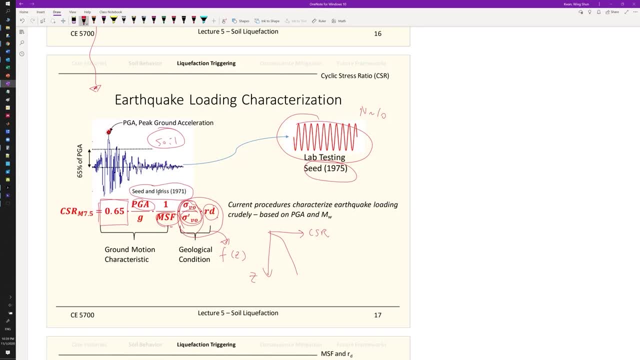 a lot of aspect of uh, of, uh, of ground motions. uh, you know those temporal uh uh differences and also, uh, the frequency differences, right? so, uh, you only use one point, you, you fail to uh describe how long the durations of grid may be and also, like you know how, the frequency content it. 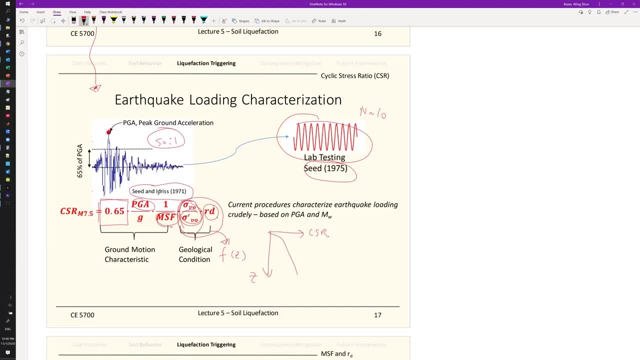 you know it could be like a soft so response that uh, you have many like uh relatively like a long period uh of uh pulses, versus like you could press stiff, sore. response that you have a lot of like small palses. they pack to each other so uh part of it you know to to adjust for the loading durations. 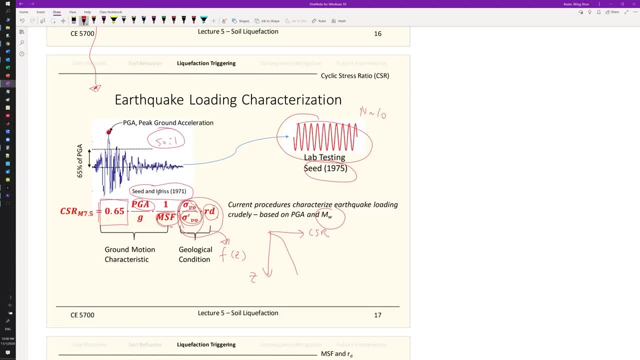 it will be handled by the correction factors of uh, the magnitude scaling factors. so, uh, we have this process called of load duration in terms of uh, you know, attractive manipulation of the magnitude scaling factor. so as much times or likely, the large magnitude scale type will be handled by check pressure over 29, shown above the slide, will be not the vessel size or whilst the vegetable size of thiserapy will not be in the same linear development, rather thanBrave millennium. on analysis, you could not look if the unemployable now you eyes, compared to a, the block size measure in general, that range of normal calibrations, no. 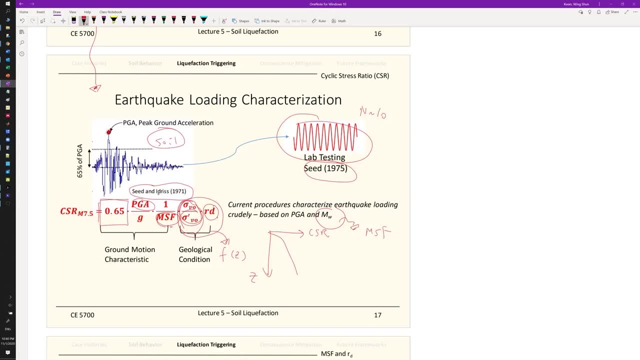 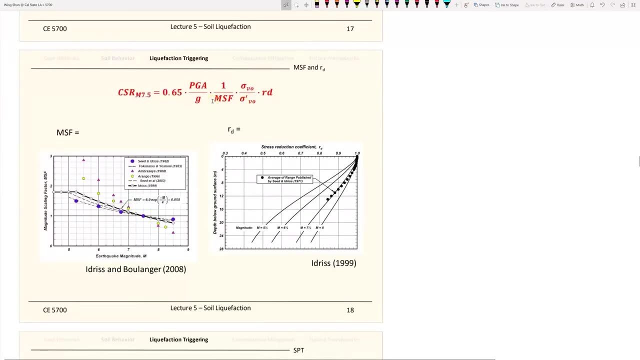 we'll talk about it next. okay, so uh, let's thirdly talk about um this trickering uh models, or trickering uh liquid fraction, trickering urination's uh framework, which is given this equations there. so, um, if you look at this equations, uh, pretty much like you know, um you we try to characterize. 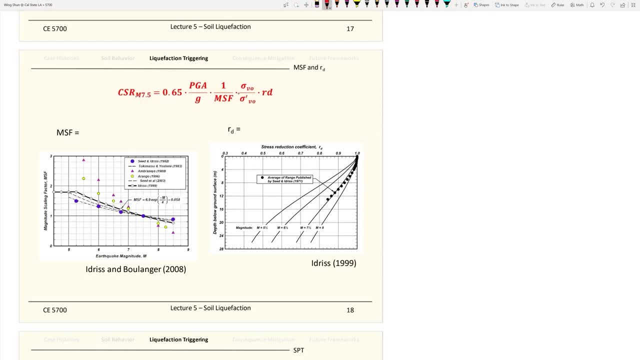 earthquake loading or earthquake ground motions by one bond, which is the pga, the peak ground accelerations, um, and then, like you know, uh, around this, um, this intensity measure, we try to correct, uh, with different, like a you know design scenario that you may have, so, um. so, you see, you come with 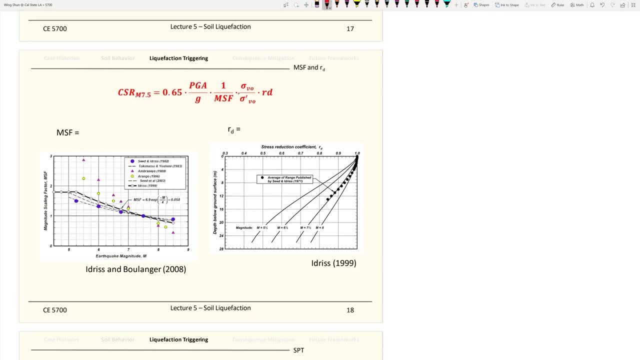 a bunch of like, a different, like uh parameters. so we talk about the original framework uh from seed. it also has the um, the total stress derived by the vertical effective stress. so you kind of like you know, take care of the uh, the open burdens or stress uh issue. because, again, 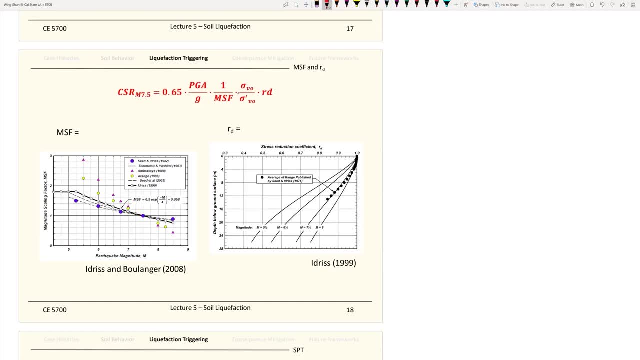 liquid fractions also depends on the stress level you're at and upon the 0.65 there is try to correct for the uh, uh, the peak, the peak ground accelerations, because it would be too conservative if you just take the maximum uh loading amortization from uh. 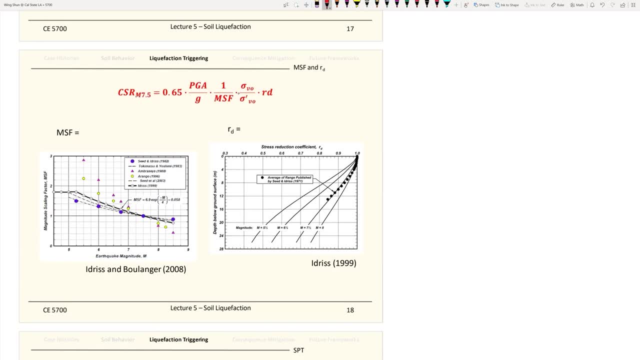 our ground motions. so, um, that's a couple correction factors to come up. uh, the first, uh talk about the msf, so it stands for the manatee, a scaling factors. so, um, the the philosophy or the reason behind this is, um, they would think, um the longer uh loading period comes from larger, uh earthquake magnitudes. so, again, like you, 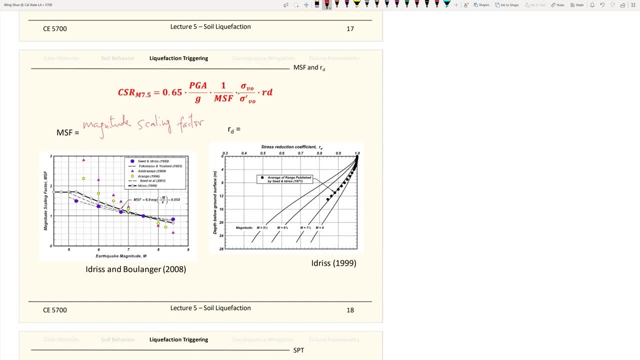 know if you have a high amplitude earthquake, if you have like a uh relative eight earthquake versus a magnitude of like a five earthquakes, uh, that would be. you could expect there would be a. there would be different like loading durations. so this msf is trying to uh bring in the time dimensions. 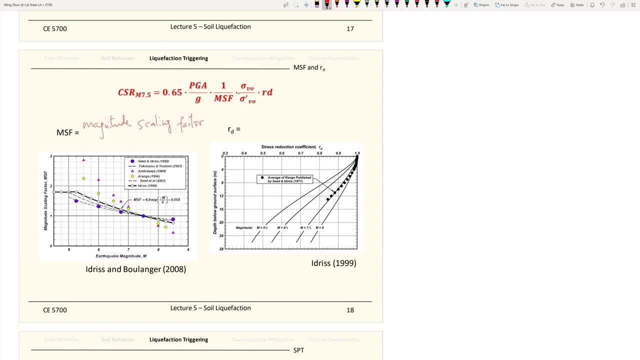 for earthquake events. you know, we know that, like, pga is just one point but like when you see the ground motions, you know you can. you can last from maybe from 15 seconds to uh, up to like a 120 seconds and using one point cannot capture the, uh, the duration, so that the time effect over there. but 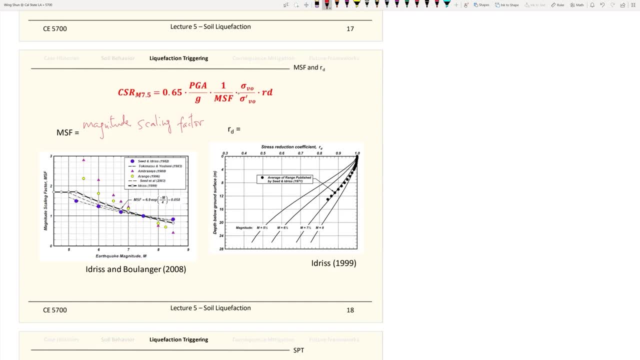 the sms. uh try to correlate with uh the durations with the mana deals. so it's very like uh rough estimations, uh, but somehow, like you know, you try to um bring in the factors. so using this mss, msf, like uh factors and this uh graph here, so you house msf factors change with uh the. 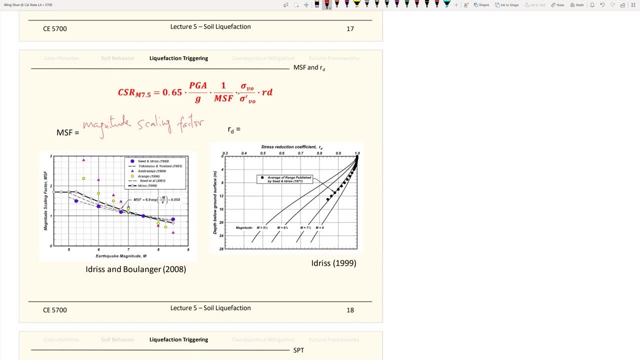 earthquake magnitudes and uh, they use magnitude seven and a half as a reference because, uh, at seven and a half, so seven and a half is here- the msf factors is equals to one, so which means like, uh, um, what they try to do here is uh, when. 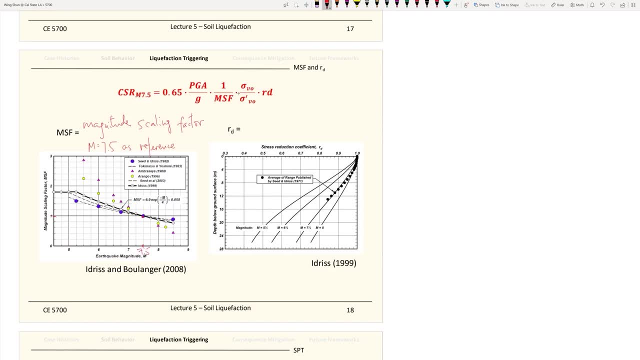 you have an earthquake uh event that is greater than 7.5, then you get a magnitude scaling factor less than one and the reciprocal of it will uh increase the, the loading, the csi of psychost터s ratios. but if you have uh earth great magnitude less than seven and a half, they 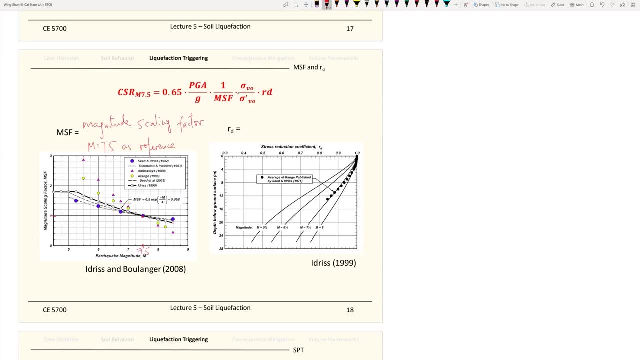 will try to penalize your earth cry loading. so seven and a half, that's the reference point and that's a bunch of different uh research done in the past. so that's why you see different, like a different data doc over there. so the eat just one and sit and interest uh arango. so uh. 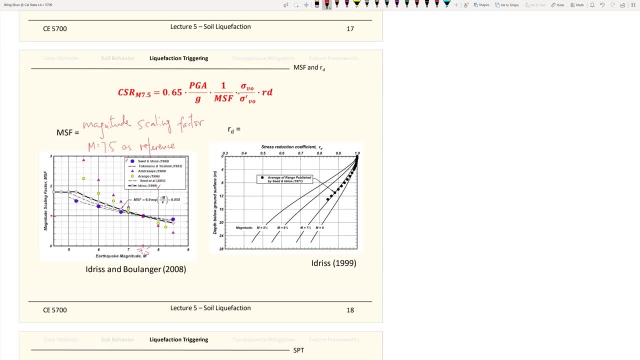 more or less. they are a little bit, uh, different, but like, uh, the philosophy behind. so you know why the difference? very likely because they have a different database to look at and with time you could, you could imagine, we have more and more earthquake records, especially the significant ones, such 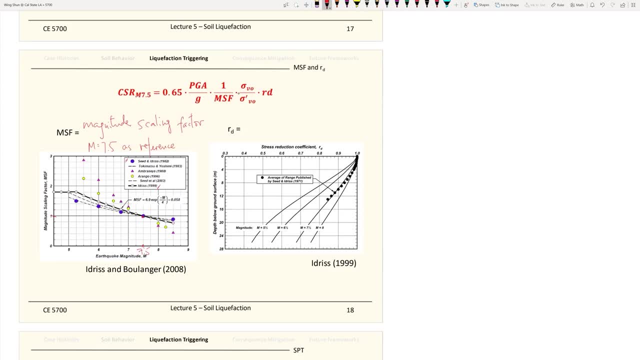 that, like this MSF relationships or this equations there will be keep updating. so you know some of the correlations over there is really outdated already, especially like the 1988 or the 1983 the Japanese one. you know, I don't think any people will be using those correlations now because one 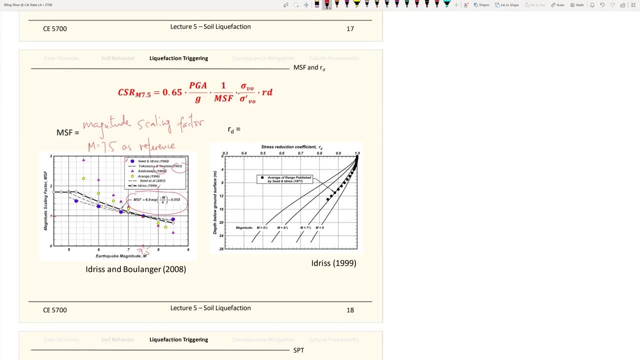 thing, like you know, some of them is quite dangerous- is even this like embossed, like a 1988 method: you go forever high and go forever low. and this may not be true because, especially for you, when you have very small earthquake and a very large earthquake. so the later developments, 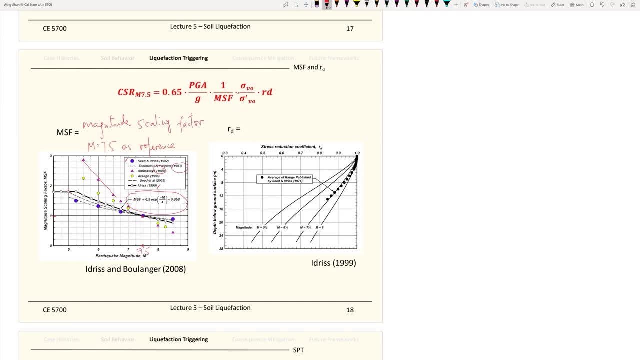 they try to cap it with more reasonable boundary as either like a very small earthquake or a large earthquake. so what I want you to get out on this is: you understand, you know what MSF- the mental scaling factor- do, and also you know- keep that in mind. 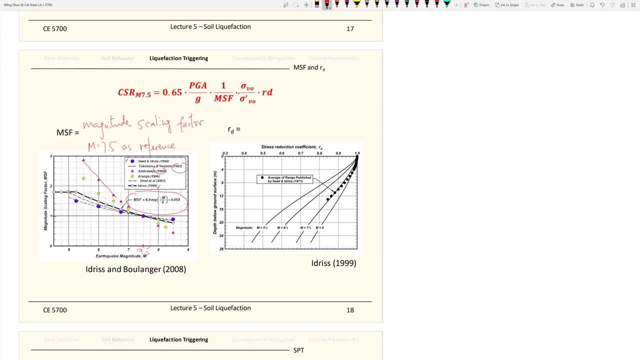 yeah, I mean there's the correlation of the correlation either to 104 and more and make it same for that quak is another strategy. it can be change. I didn't showới the corr all this stationary curl will do. but the one thing that makes sense is when we look at 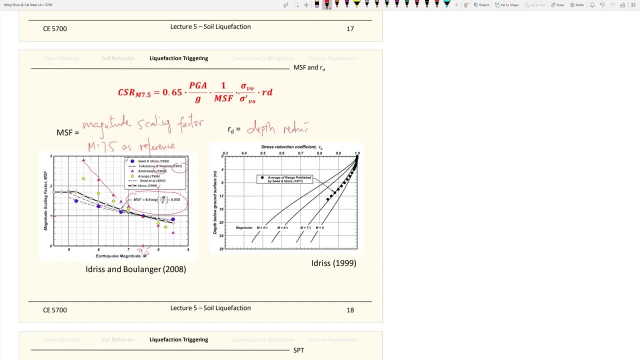 those correlations or those factors we will be updated from time to time, especially, like you know, where we got, like a more and more significant data for recent earthquakes and the air. the other factors is the death reductions practice. so dep직 of having this assault D over there is is probably a little bit older to have so for the purposes of halt titles over there is to have this out sub D over there is his own Asian afterall, nine years of time now because, unlike Quran, was to get that facts for strange stuff for counter borders onlyを. 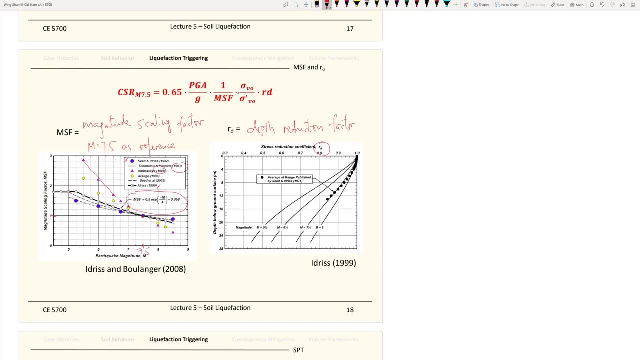 Is to correct for the liquid fractions triggering with the depth, because the deeper you go, The less likely like liquid fractions will be happens. So liquid fractions is a phenomenal that happens at. You know, the shrivel ground With a depth if you get a great, really great depth. 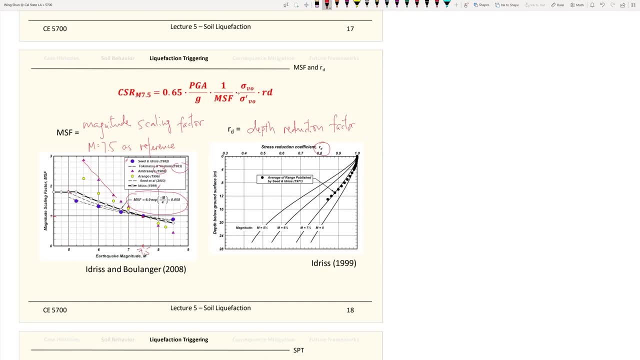 I don't think, I don't think like liquid fractions will happens, because the confining stress is so high that, If you understand this, if you truly understand, like a critical state soil mechanics, The dilative behavior of soil Depends on both density and also the vertical stress, the confining stress. 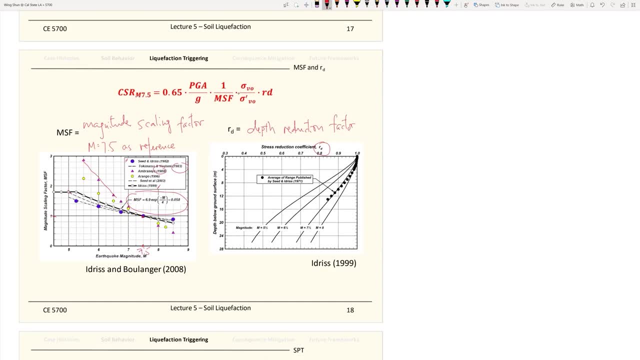 So when you have a very high confining stress, no matter what density you are at, Very likely you will have a dilative response versus a contractive response Of of the same behavior. So when you have dilative response, you're generating Negative excess pore pressure, which will increase your soil strength rather than decrease. 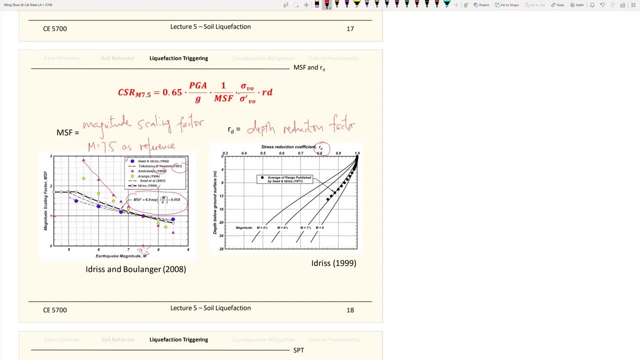 so you may have psychic mobility but you know your loading and also your Loading durations may be, may not be strong and long enough to Move past the psychic mobility to the full type of a solid liquid fractions. So those are the two factors and again, like at this ounce of D, like the MSF, scaling factors. 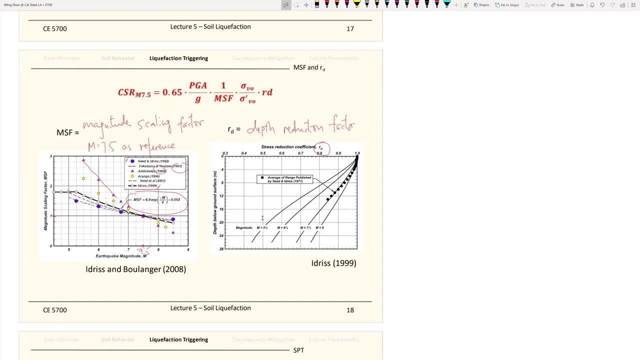 From time to time those correlations will be updated because again we have more a data to kick scene and those Informations or those correlations will be changed. So If this is like a very fast evolving, You know, engineering business, unlike the geotech, the traditional geotechs, that 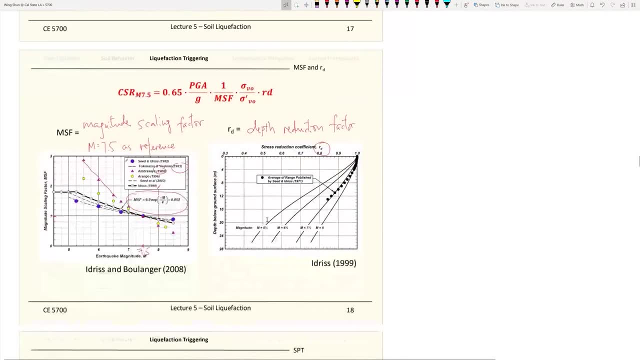 You know everything on the statics and you know whatever We find out in the 60s, the world didn't change much. Are you still living on earth? and you know. So the framework and the analysis, analytical approach is still valid. but for earthquake engineering, you know every that case thing will like. you know we have a. 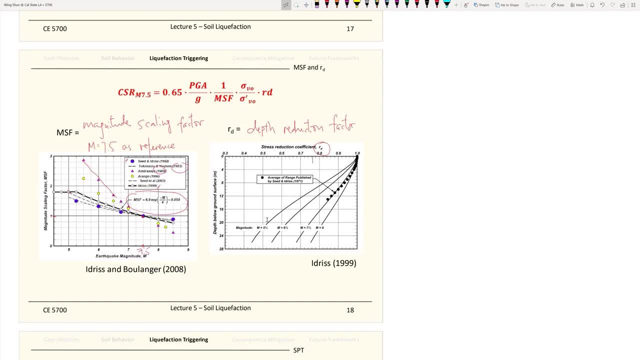 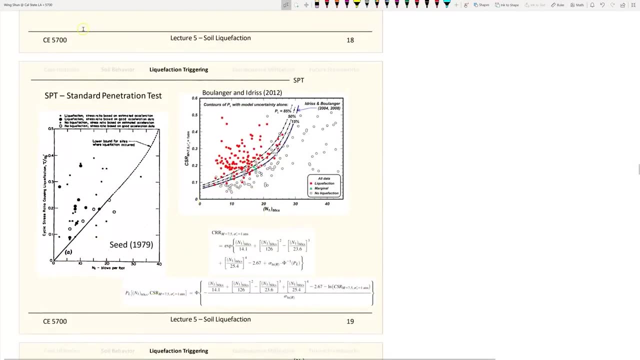 New generations of models has come up, So is you need to pretty much keep learning if you want to stay in this business. So this slide gives you an idea on how we establish the SPD based solid fractions triggering curve. so So this is the our solid correction triggering curve, right there. 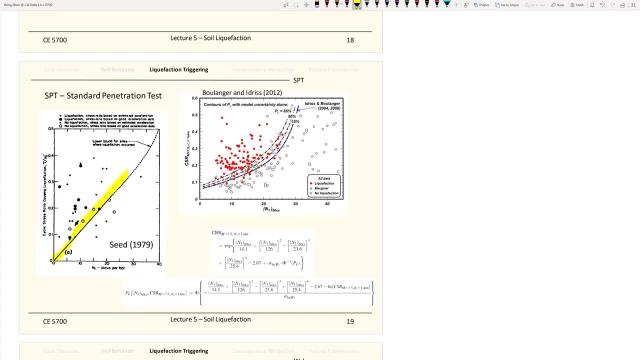 So pretty much like we use this for design and this is the very first one from our 1979 come up from seat. So how he come up with this, pretty much like the x and y axis. So the x-axis you can think of is kind of like the loading. 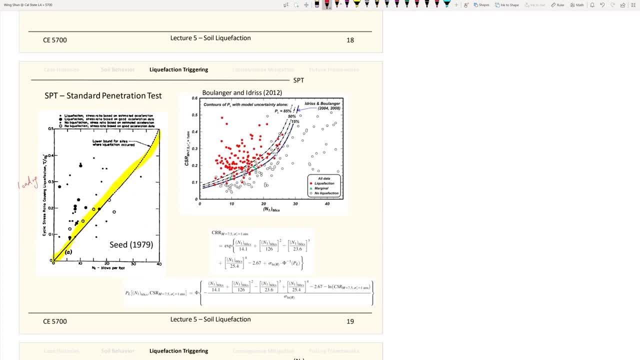 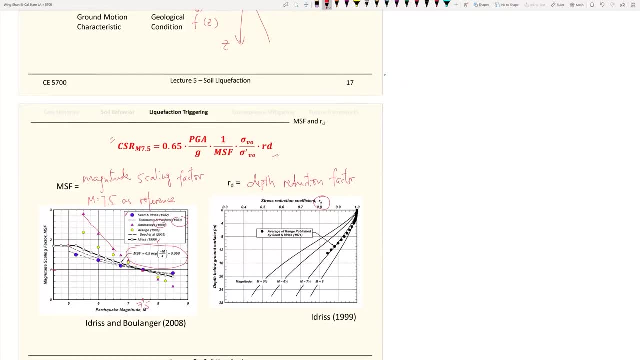 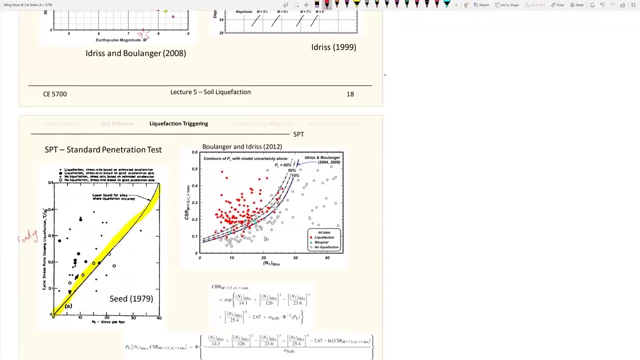 So he calculate the psychic stress ratios, very similar to To what we have on these equations, but back to the old days. He have a more, even more simplified framework. So pretty much just like a convert, like maybe a record to a shear stress time history using new griffin's means. 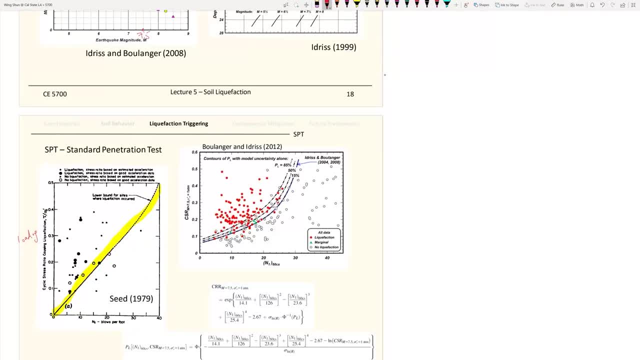 You griffin's like a such response Analysis and then divided that by the vertical stress, so even like a, not bother with the mental scaling factors and also the the depth reductions are factors. But that was the old days. but the concept here is like you know from each K history. 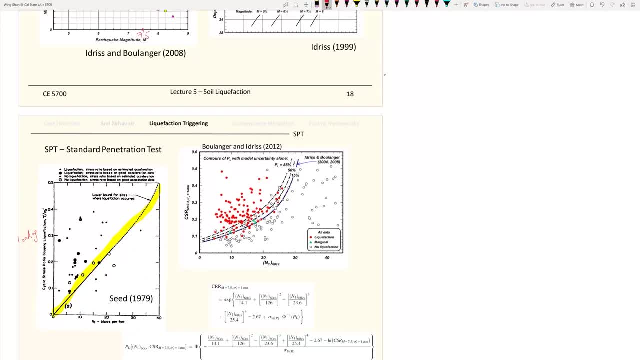 So each data point, there is a K history. So this could be like the San Francisco earthquake, This could be the Japanese Coyota earthquakes, this could be the the Taiwan Chi Chi earthquakes. So I'm making, I'm making that up, but, like you know, this could be the 1999, that's even before 1999. 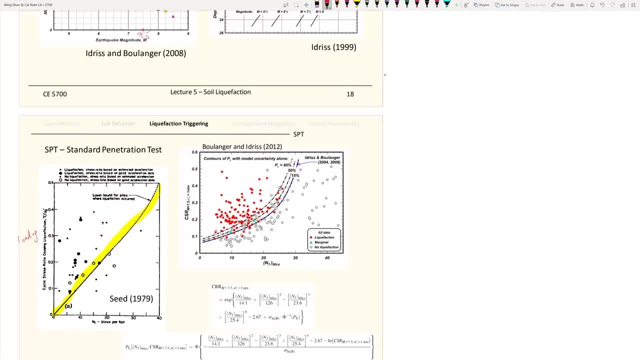 So 1999 has a very famous Earthquake at Turkey, the Kujari earthquake. But anyways, like you know, each data point represent like earthquake records and then he back calculate the loading and then you find, Like this on the site you find it- the SPT data. So this represent the resistance. 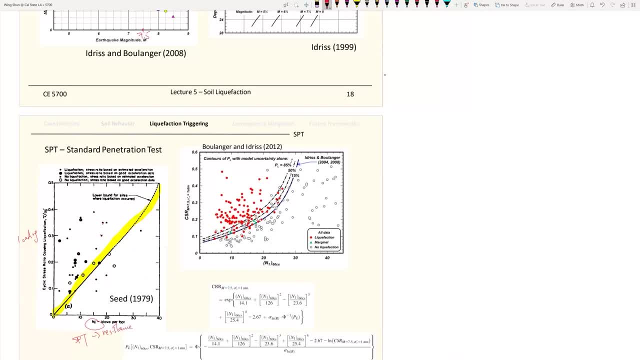 So there's always system represented by SPT blocon and then, like he has the, the binary classifications, where the like the doctor, one is the where liquefaction to be happens, and The open one is like a there's no liquefaction Happens. So remember, we watched the YouTube clip together. 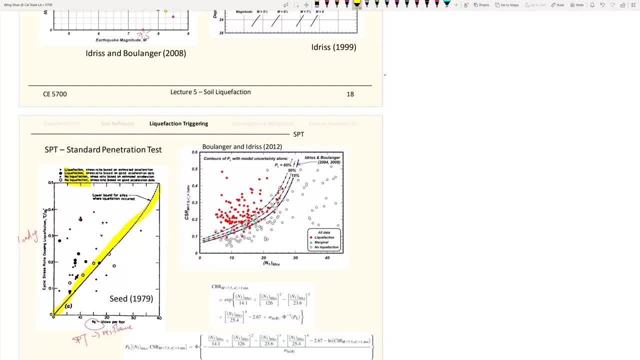 The evidence of like a fashion see, see whether you see the sand, sand boiling on the sand, That effect way they can trace the excess pore pressure being shut off from the site. Then they can. that they will. they will know like a red the liquid factions happen or not. 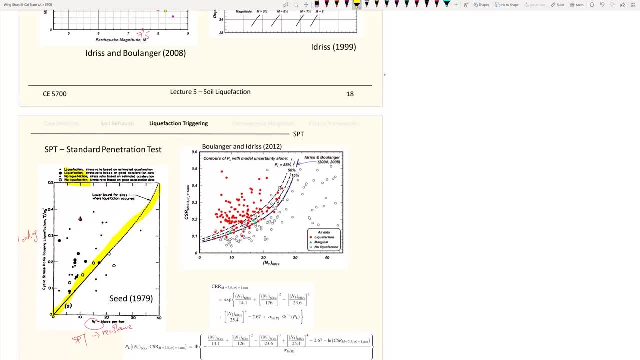 so if those destinations they can draw, try to draw a reasonable binary curve. so we call this the liquefaction capacity curve and That apply this like kind of like a worldwide for design. so you've, you know your SPT, then you can have a quick estimate. uh, you know your spt and under also you know your uh, psychic stress ratios, then 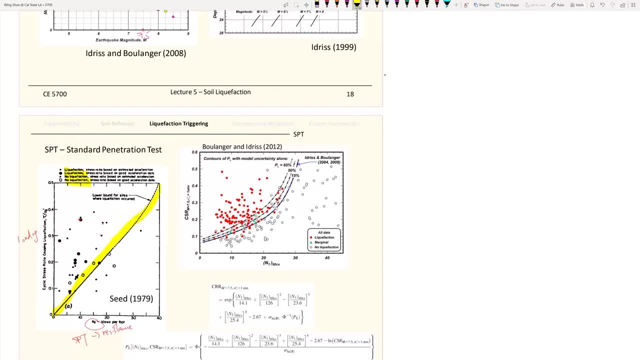 uh, we, you can have a quick estimate uh, whether, like you know you should expect this sort of factors is tricky or not. so that's the spt of the old days and uh, i have one that like are quite uh, uh, quite used oftenly. so this even is not the most updated versions, but like, uh, this is our. 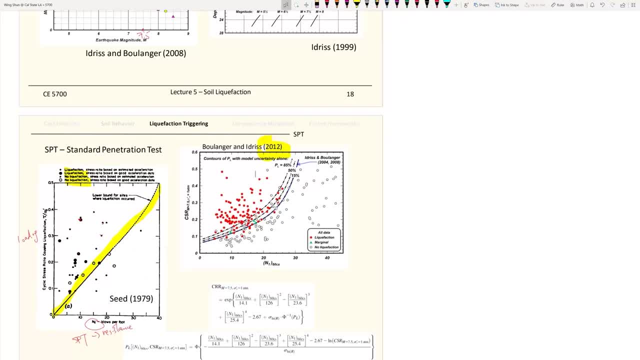 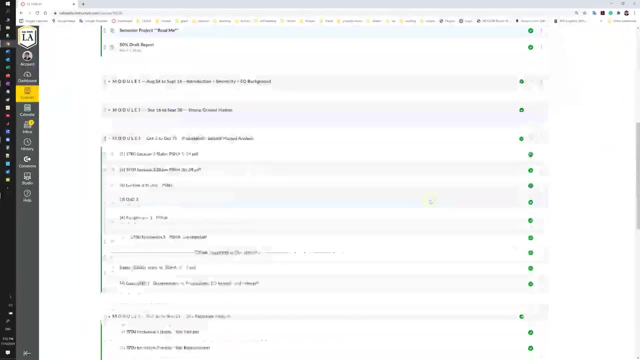 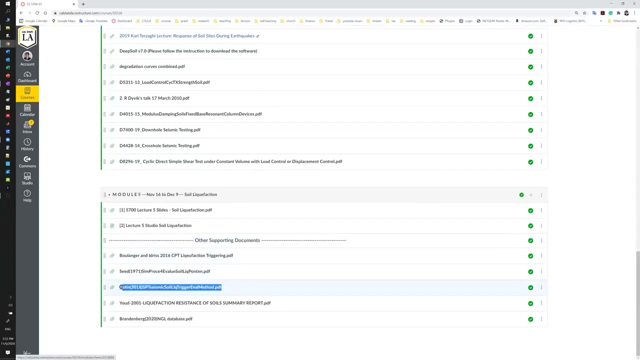 recent work that, like uh, been well organized and i updated, i'm sorry, uploaded two papers on uh, on camfax. so if you go to canvax, go to five, seven, zero, zero. so if you go to camfax, um uh, the most updated one should be the seton uh 2018 method. so that is um, the most updated spt. 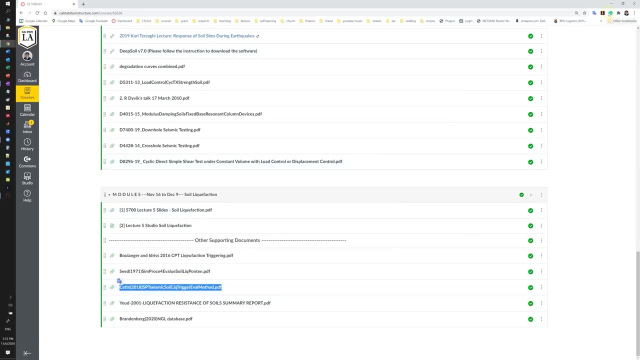 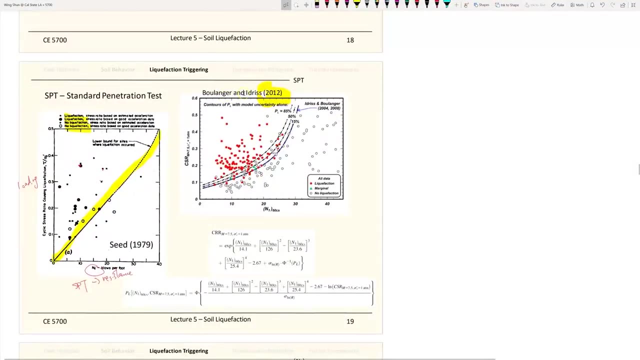 method. it for solid liquefaction triggerings and for sure, like you know, i think, sedans. he pretty much like you expect. uh, he built on blanc j8 just like a model, so, um, so you can see the difference between, like a 2012 and 1979. uh, you have much more data points now and uh, the red docs means, like you find. 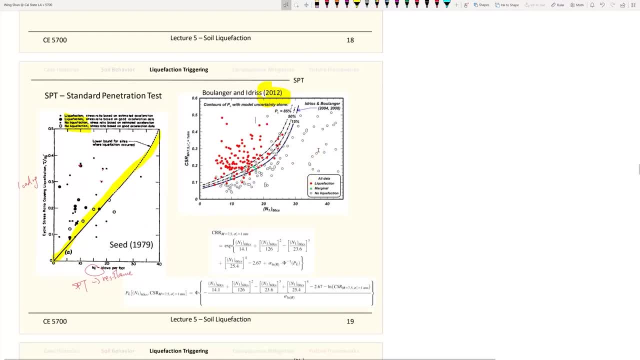 the uh liquefaction's evidence, the open doxes? you don't have it. and um, now, nowadays, like uh, uh, deterministic analysis, um, you know, we try to move, move past that. uh, we, we adopt more probabilistic approach. so they even give you um three different probabilistic uh capacity curve. 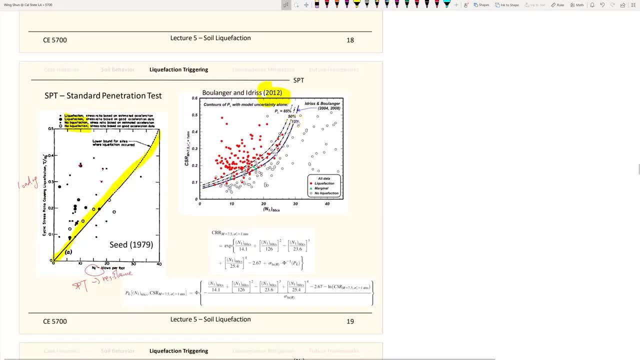 right there. so 15 of like a likelihood for liquid fractions to be happens, or 85 percent of liquid fractions, uh capacity curve of uh for. like you know, uh for for that being triggered. so it can be uh expressed in terms of probability and um, here is the their probability model. so if you want to, 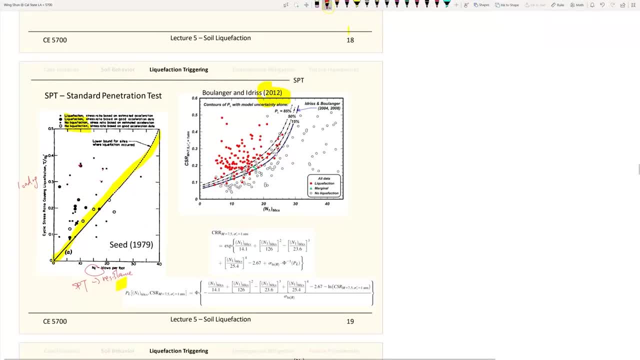 call it uh. if you want to develop your own uh computations like a program or your matlab or excel spare heat, you can use the code here. but if you want to do a quick analysis- uh deterministic approach, you know, somehow you you bring in some probabilistic uh components right there, you know. 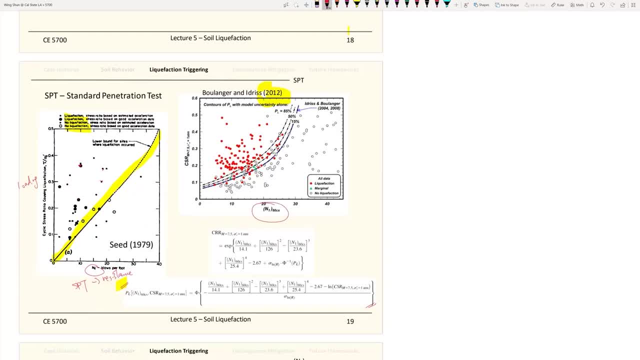 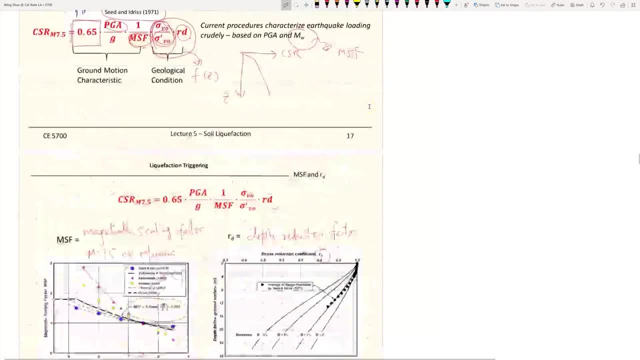 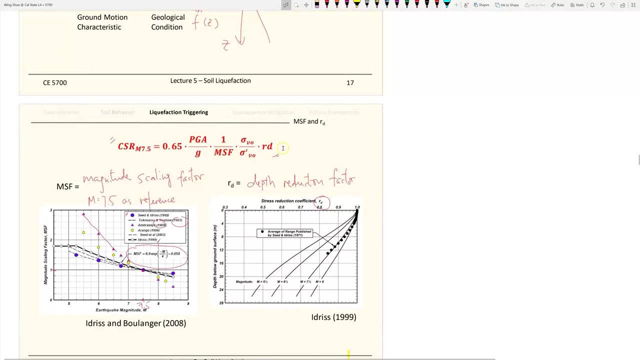 you can just read off the curve, so so, so all the corrections are there. the m160 clean sand and this is a truly compatible with the csl right here that we talked about. so you, it has already correct for the magnitude scaling factors: uh, the death, uh, factors, so, um, you can't, you calculate. 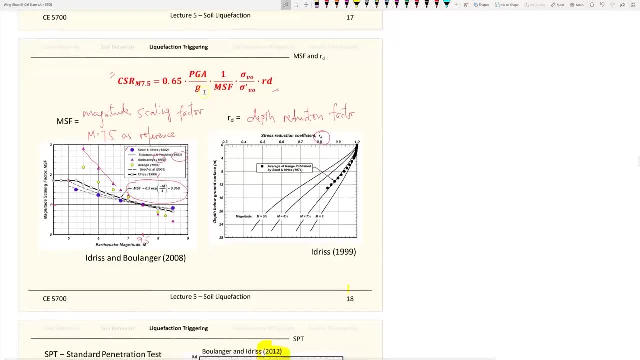 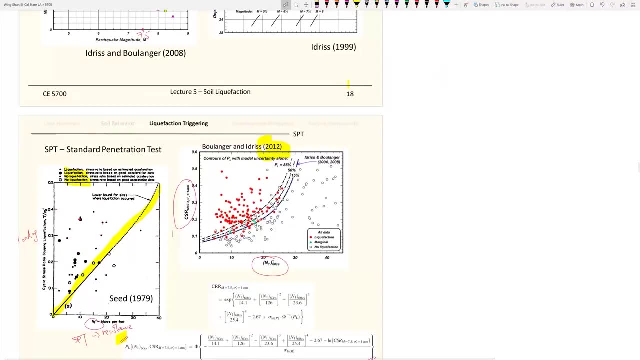 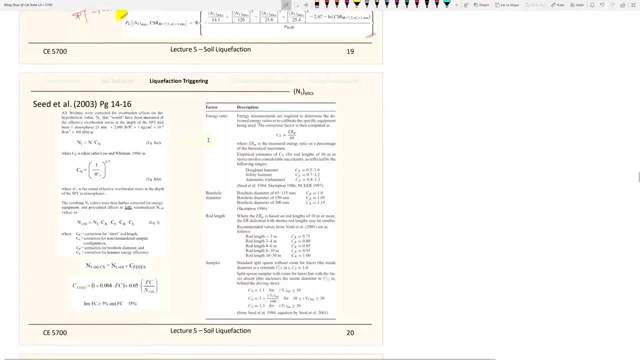 through this trick, triggering a solid liquefaction, triggering equations, so you get the y-axis, you know the loading and then compare with your corrected spd resistance at the end blow counts. so that is the spt approach and for more information about uh, how to calculate the n160. 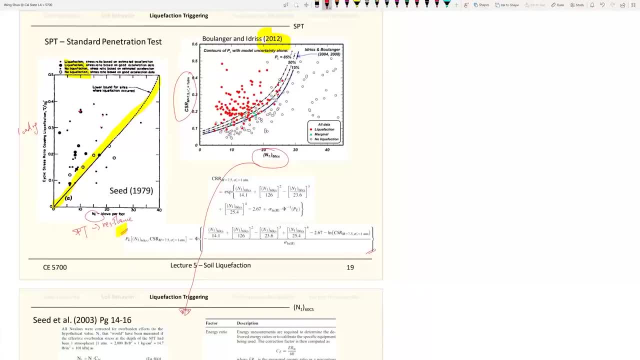 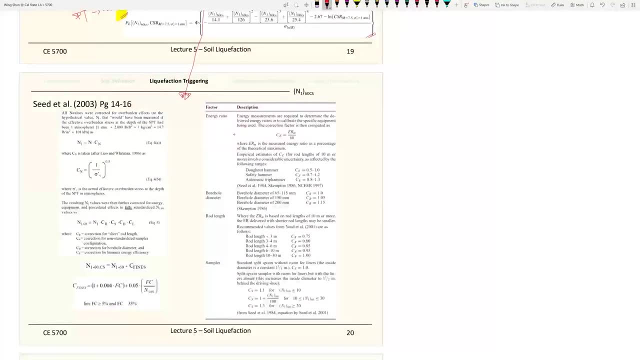 there's like a seat, raymond seat, not the harry said so. the younger seat, the seat that's junior seat, uh, you know who, who just retired, even though, like you know how, the junior seat, uh, he retired, i think, a couple years ago, from berkeley, but this is his work, uh, in 2003. so he gives you at least. 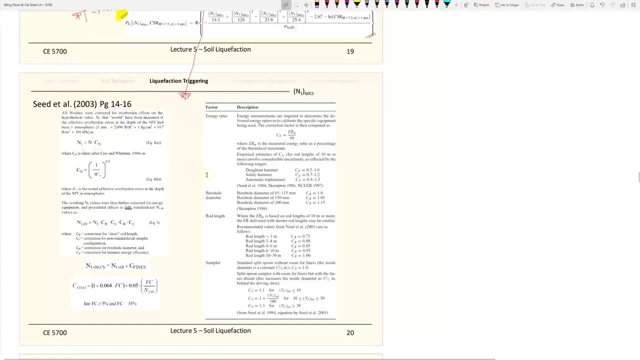 or he can walk you through how to correct the uh sptn values: from uh to add n160, clean sand. so uh, just give you the details and how courage you read the paper. uh, there's still a lot. 2003 paper. you may be a little bit out of date, but 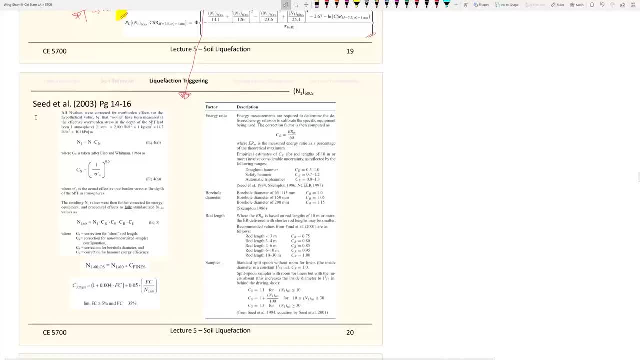 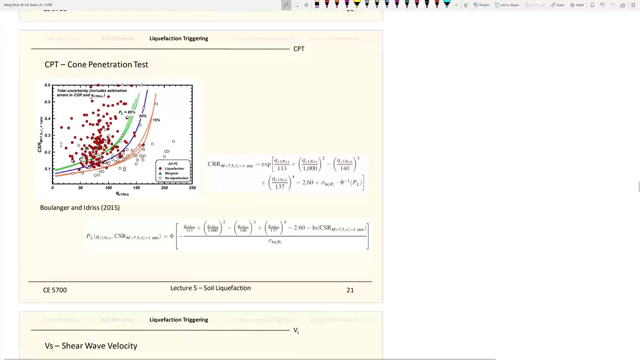 um, i think seat uh uh. professor raymond said he did a good job on uh explaining uh the, you know the the overall design procedure uh in the seat 2003 paper. so, um, that's a spt approach. likewise you also have a cpt approach. so if, if you do your site uh site investigation program with cpt rather, 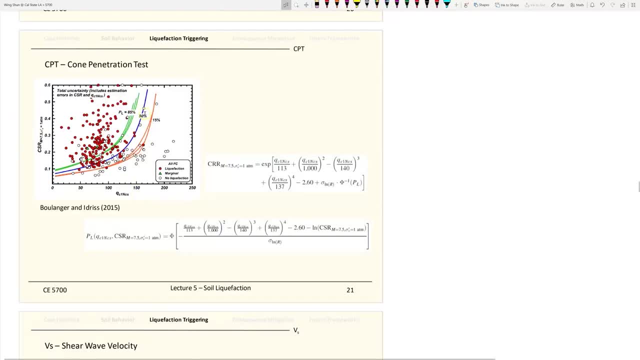 similar concept. uh, you have the uh uh the probability state. uh, solid fractions, triggering capacity curve, right there, uh again like a boulangerie, just a uc davis, they did a lot of good work, uh, they both uh. so it is kind of like uh the very uh two first two students of uh uh. 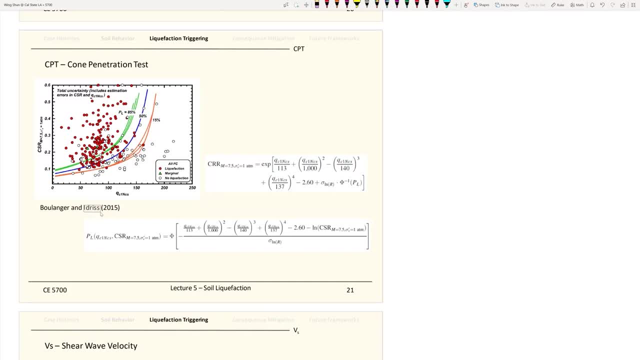 the, the famous heavy seat at berkeley, i think back to 60s. uh, and then, like a boulangerie, is, is, uh, it's all. it's the last, uh, almost uh, the last students of, uh, uh, uh, dr harris seat. uh, in the. 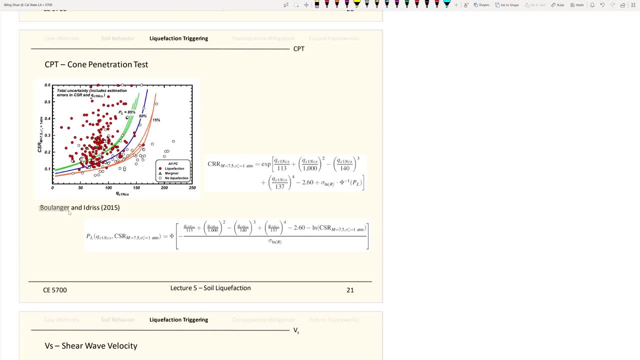 late 80s and early 90s at berkeley. so, uh, even though, like i think, uh, uh, dr harris, professor harris said he passed away in the middle of dr boulanger's phd study at berkeley. so i end up like dr boulanger's uh, uh. dissertation is signed off by the junior seat. 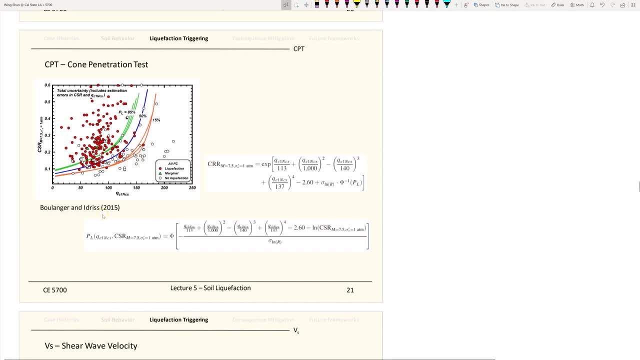 but anyways, uh, so, uh, they somehow, they, they, they both become faculty at uc davis and they did a lot of good work on uh in the topic of solid group fractions. uh, so, so that's why, like you know, in california, and also, um, uh, particularly in the geotech earthquake, engineering like a business. 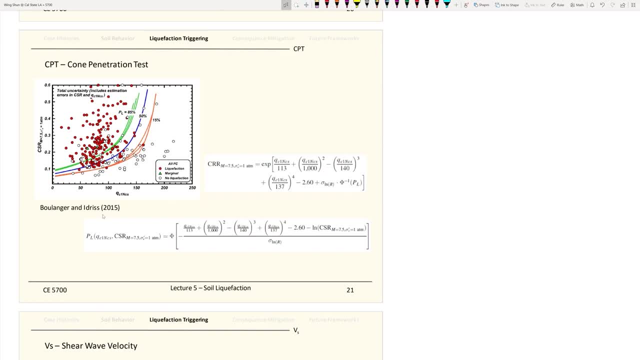 is strongly you for, influenced by by uh the berkeley grad and again the textbook that uh you read uh from steve kramer. he's also very important uh players, or importance like contributors and in all this subject, as well as like dr jonathan, professor jonathan jonathan bray, and now who is? 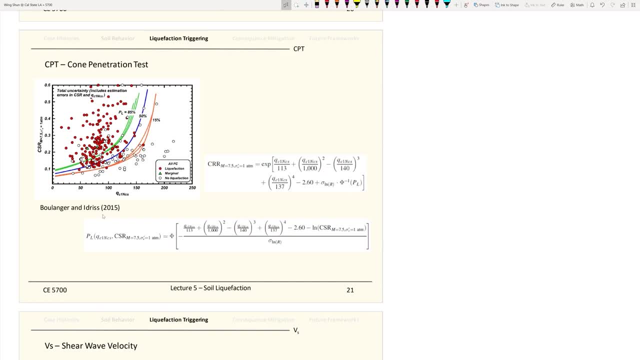 still working at berkeley. uh, he is again one of the last students of uh, dr harry seed, but anyways, um, so this is the cpt, uh framework and you know all this um probabilistic capacity curve and if you know the equations of how to come up with those curve. so this is the spt. uh, uh, sorry, the cpt. 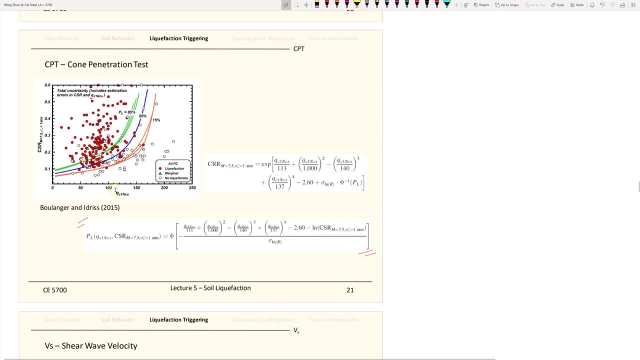 probabilistic capacity curve. so, again, if you know your cpt values, like you know uh, this chart demonstrate uh whether it's still, like you know, a cost of uh binding reclassifications where, like you're, above uh the curve is liquid fractions expected to be happens below the curve is. 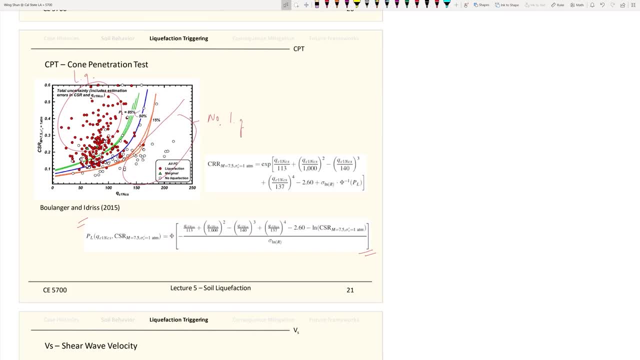 uh, there's no uh liquid fractions and you between all those are kind of like the marginal case. so you need to be like, for sure, you need to have like a third uh examinations, uh whether, how likely uh liquid fractions will happen. so if you uh fall between those, uh, you know your design scenario. 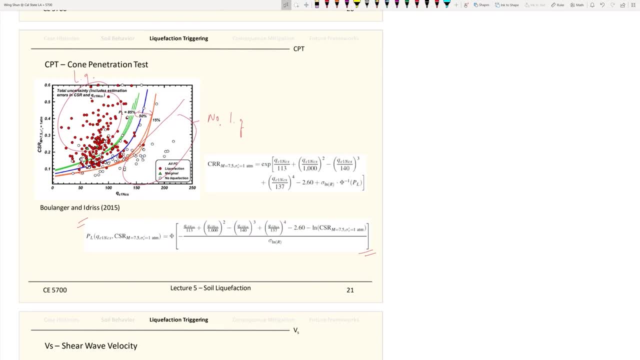 based on loading and resistance for between, like the, the red and the blue, uh curve, capacity curve. you know, those are the most difficult uh, uh analysis or decisions that uh the engineers need to make. you know, uh, rather, you should, you should, you should treat it as or you should do a ground. 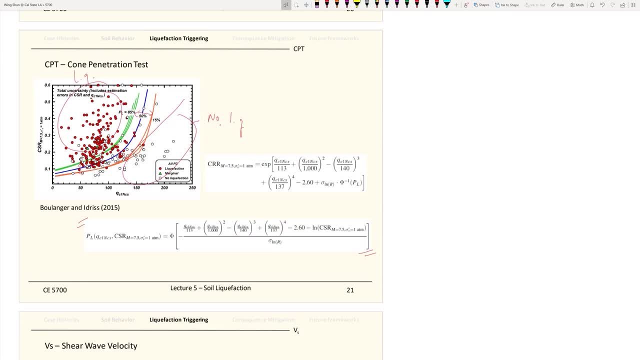 improvement to avoid uh sort of uh, you know solid reflections to be happens. uh, if you, if you, you know if your design point is out here or right there, you know you make a choice easy. you know for very likely, you know nothing is such it's 100 sure. 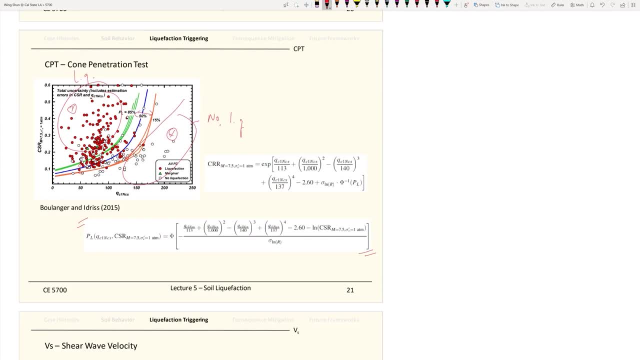 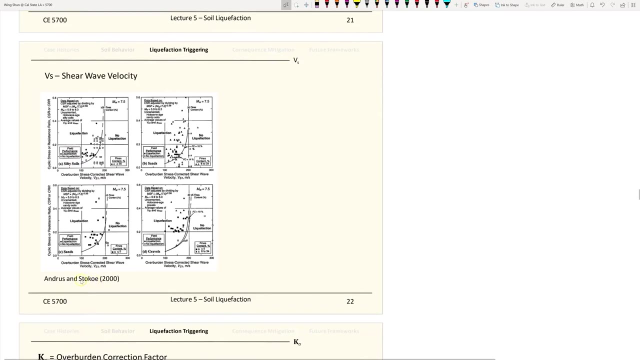 reverse earthquakes, uh, design. but you know you have some sort of certainty when you are far away from those curves, but anyways, like this gives you an idea of how the cpt works. and uh, likewise, um, as a stokey at texas, you know, he's the one that, like one of the, the anti-berkeley camp. 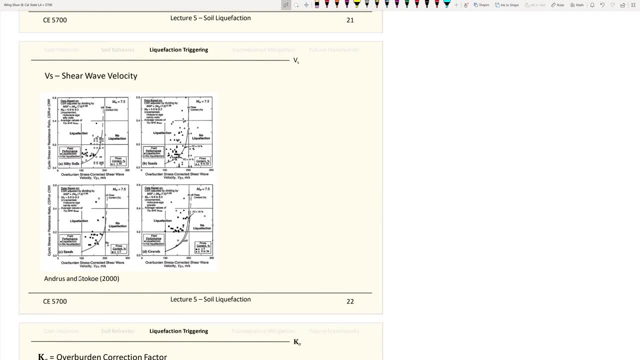 so, uh, earthquake engineering, uh, you know the geodetic earthquake engineering at some points, like you know, uh kind of like divided into two parties, you know a little bit like our country now, uh is the berkeley camps versus the rest of the world. you know could be the texas people. 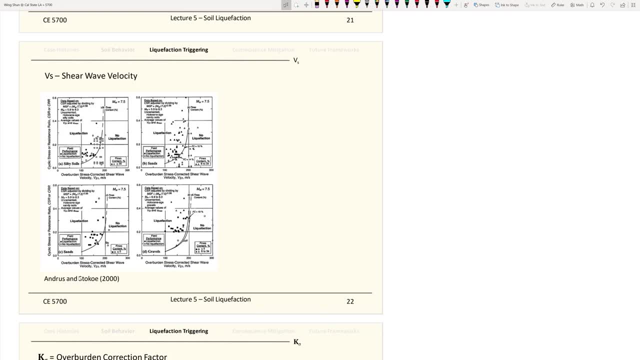 and also the japanese, like uh scholar. uh, they have different views on how to uh look at this issue and then, uh, they come out with another approach. uh, instead of like a last strength behavior that you use sbt or cpt, uh, they truly believe. uh, the soil behavior or the dynamic of assault properties is dictated by 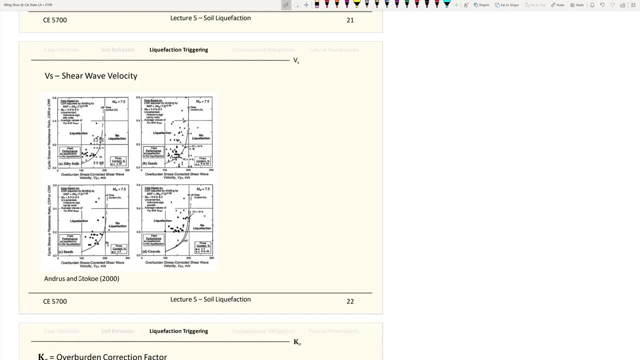 uh small string behavior, which means like: uh, they don't buy into those destructive geotech investigations or geotech field index like cbt or sbt, but they more have put more like a faith into uh small string parameters like the shear string, uh shear wave, uh velocity, which is small. 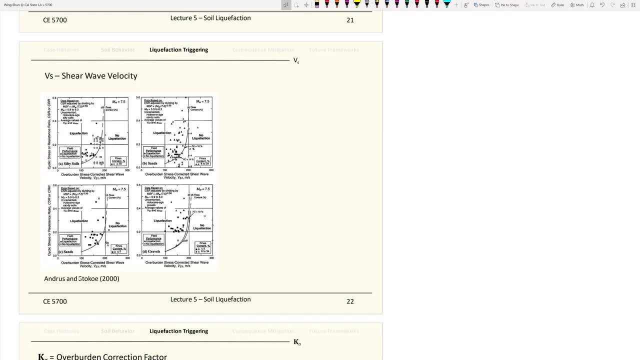 string behavior, uh, small string measurements, like you know, the cost hole and the downhole we talk about in the soil, dynamic dynamic saw dynamic properties lecture. so, again, like you know, uh, so dr stokey at texas, ah, andrews is his circuit students, so he come up with those again, like the. 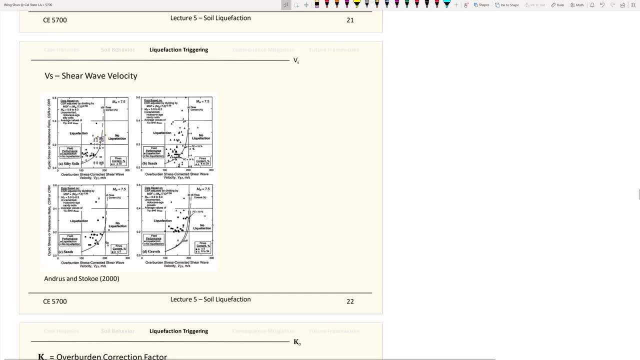 triggering curve us. so so look, reflection capacity curve. uh, divided the data that like they, they find the versus no electrification and then depends on different scenario. you know those are the uh, the shear wave velocity curve, which is less uh common in practice, uh i, i guess one of the 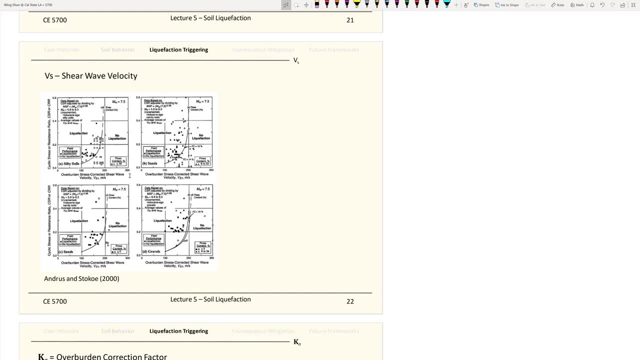 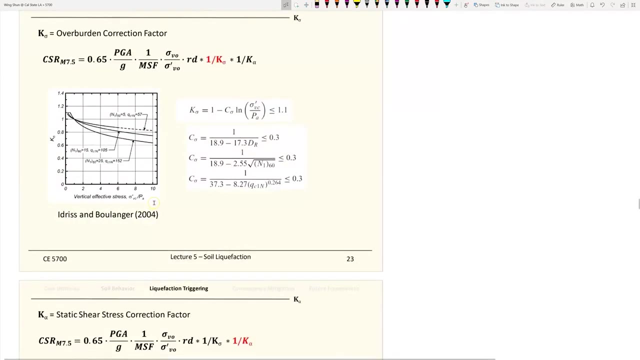 main reason is it's not cheap but it's not common. you get uh shear wave velocity measurements wanting those crossover downhill tests. it's more common, you know, commonly available for those spt and cpt investigations. okay, so, uh, building up on the csr stress profiles, uh, we have two more. 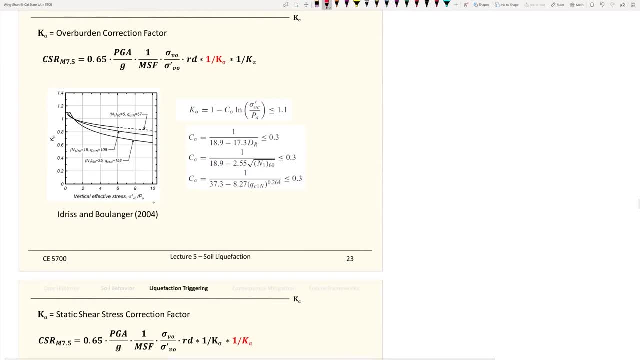 correction factors that i want to talk about first is the case sigma, which is the overburden correction factor. so this is correcting the overburden stress, a little bit like the death of reduction effect factors. so this correction factors pretty much is um, this helps you to uh, to change to, you know, to penalize uh the loading or to reduce loading when. 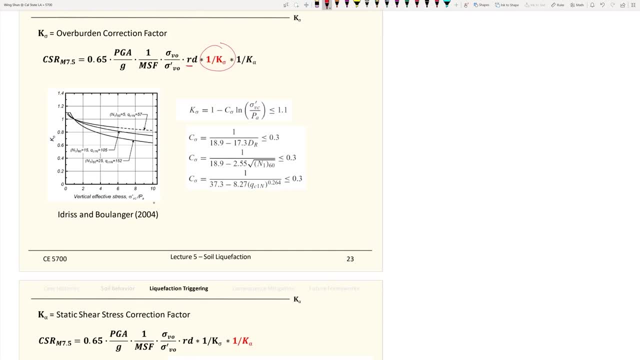 you're at like greater depth, which means like higher, higher over burden stress, or like uh. when you're at more shallow ground, when you have a lower confining stress, you will kind of like: pump up the loading, increase the loading. so that's um, and they use like a. 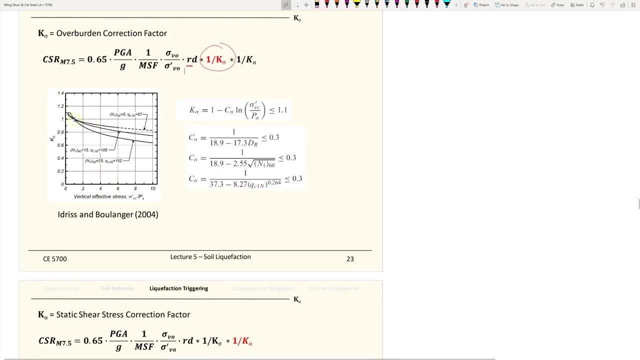 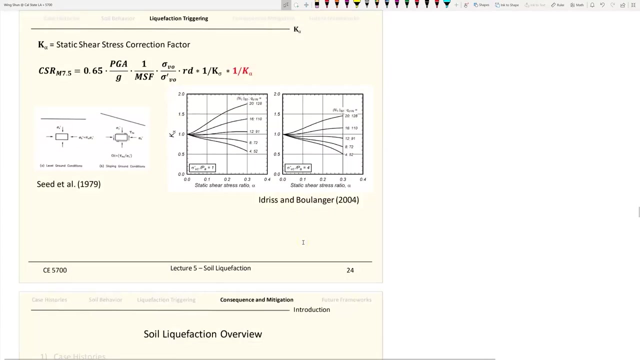 180 m or uh, as the reference point right here. so piece of eight over there, seven for a one, as both static pressure. so which is uh? so this is uh. one atm equals to, uh, the 2116 psf. the other factors is what we call this, a static shear stress. uh, correction factors. 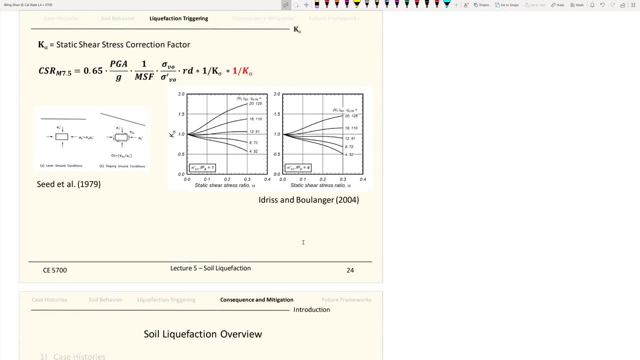 uh. so this one, uh, is a correction for kind of like a sloping ground. so when you have a sloping ground conditions, uh, that's kind of like a static shear stress adding on soil. so this is very complicated and you know, a lot of like research still need to be get done in this subject. uh, in the past, 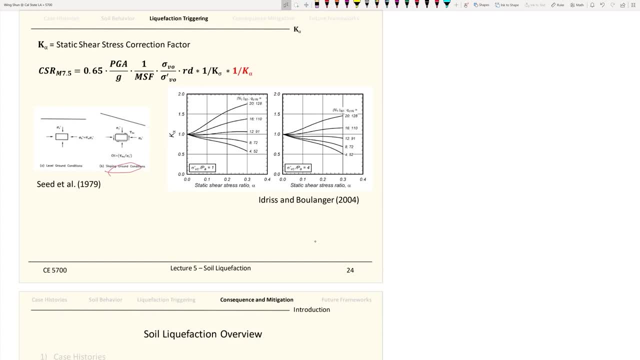 two decades, i think, like you know, this was the of the interest on the research communities on how to tackle this, uh, this problems, because, um, liquid fractions in a free field again, which means like, uh, just like, kind of like an open ground, it's likely not our interest, right. 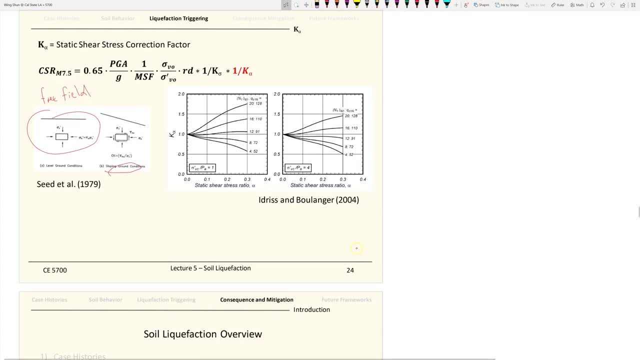 because, in urban settings very likely, uh, you have, uh, pretty much your spot, your site. you do have a building over there and your building will be imposing a static stress to your soil elements. so you're feeling this huge stress on the elements, that's our elements. so the sloping, 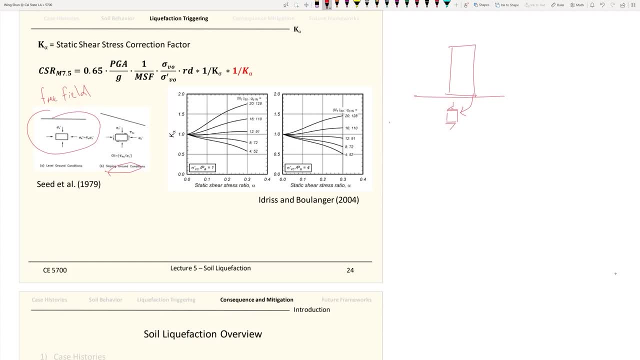 one is is one kind of like a more simple loading adding on your soil that is uh suspicious to uh solid reflections triggering uh. you'll be even more complicated when you have a building. you have structural loading sitting uh on your on your project site. so where, like, you want to investigate the uh, the triggering solid group fractions? uh, in fact, like. 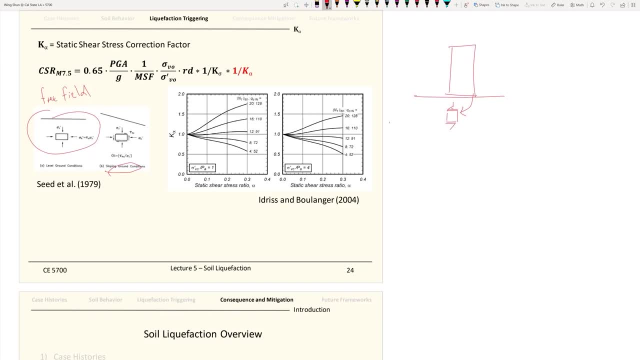 uh, dr jonathan, professor jonathan bray at berkeley, and you know, focus on this subject which is, uh, try to develop engineering procedure to find out, uh, uh, the effect of like structural loading on liquid fractions, like a trigger right. so it's quite fascinating. you know you need like a very 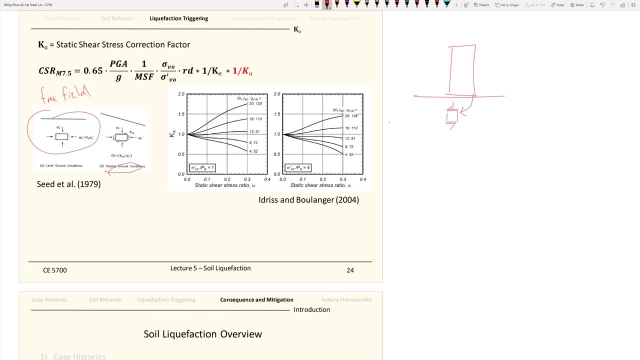 compact like a 3d modeling. so to look at those issues so pretty much you need to use like, uh, like a program like flash to help you when you get get there the effect of the structure and i can know again. if you want to learn flag, feel free to take the, the foundation of the, the advanced geotechnology site course. 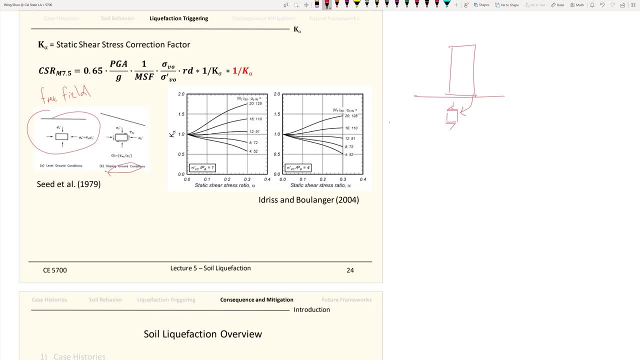 that we offer next semester, c5670, but anyways, i got the liquid fractions, uh issue here. is all this a case of alpha, the, the correctional factors, is try to uh correct for the um, this ground, you think of that, this alpha values is this equals to the, the shear. 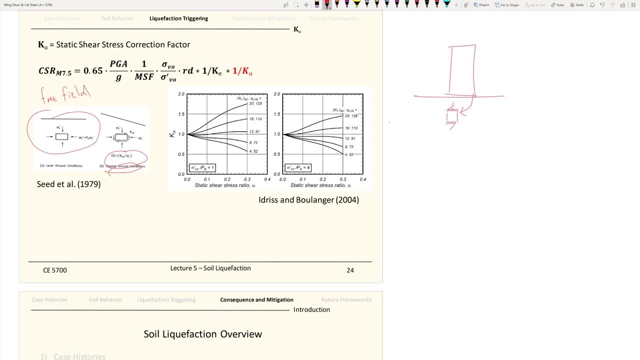 stress divided by the vertical effective stress. so if you know your alpha values and then, like you know, you know your m160 or Q CPT values, there you give you an estimate on what kind of case of alpha should you should be using and you realize actually there's quite a lot of uncertainty when you go and you use. 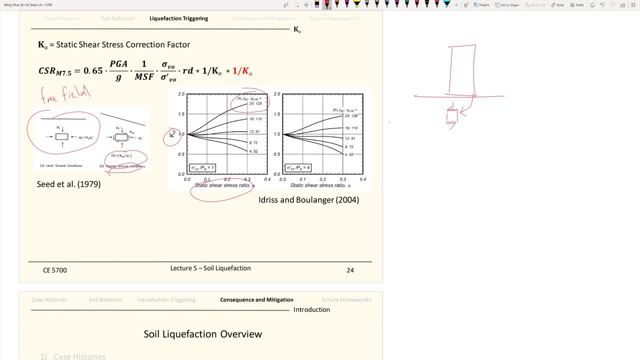 those parameters and I put out those graph from the very original work from just and belong J and I. you know, I bet, like you know, from time to time you know this- this kind of case of alpha will make some minor change, so you need to keep an eyes on how this case of alpha being changed, like you know, with